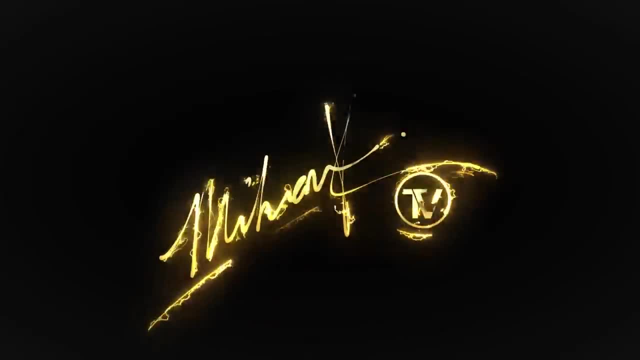 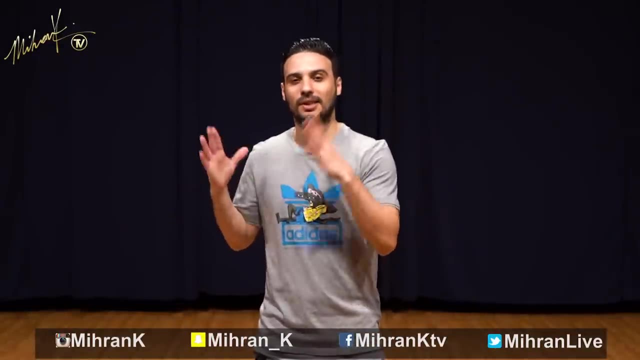 What's going on YouTube. Welcome back to another tutorial. My name is Miron Kirakosian. Today we're going to focus on an easy beginner kid's routine to the song Seven Rings by Ariana Grande. If you have not seen the dance video, I'm going to put a link in the description. 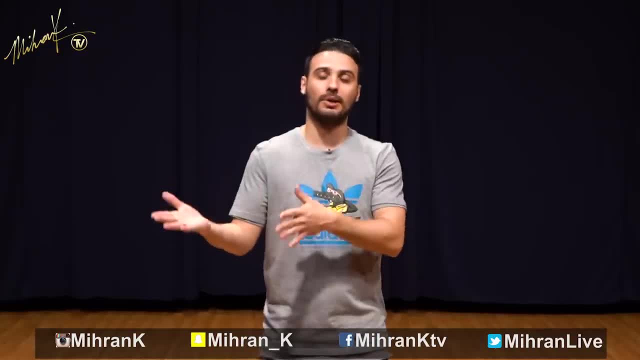 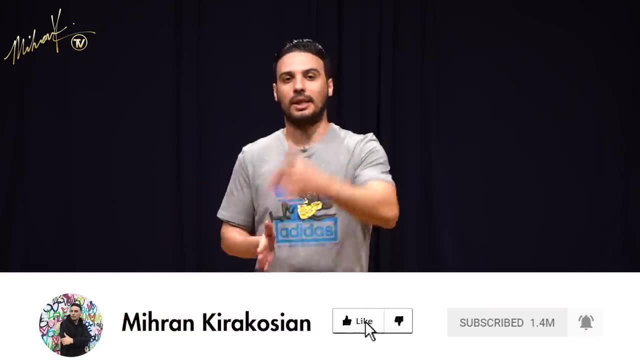 box. Make sure to check it out. Also, before we get started, I want to let you know if you've been on this channel. you've been watching the dance videos and the tutorials and you still have not subscribed. please subscribe. Make sure to hit that like button and also. 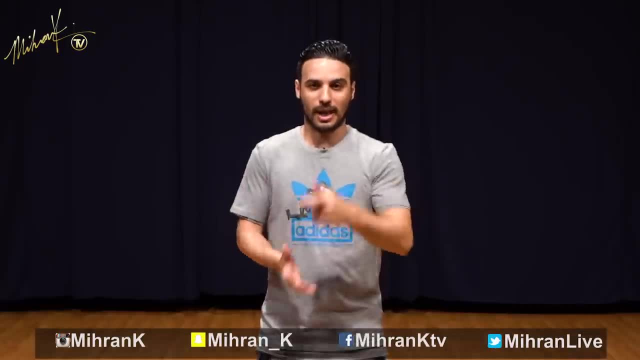 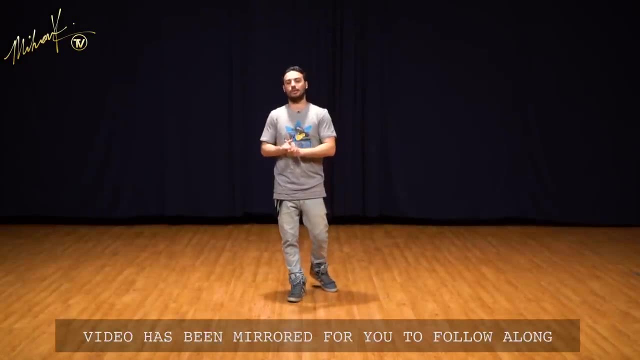 hit the bell to get notified on all the releases. Let's not waste any time. Let's get started. Like I said before, this is a beginner routine. The steps are pretty easy. We're focusing a little bit more on timing now. You just want to be sharp, You want to be on the timing. 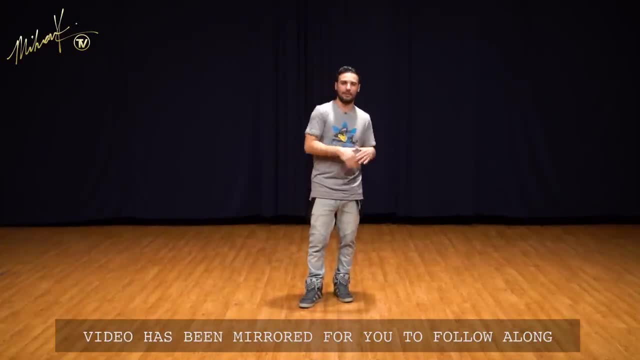 It's not going to have your basic regular timing on a beat. We're going off of the lyrics as well. I'll try to teach you what the lyrics as well- and what the counts, so you have an idea Right from the very beginning. we're sliding over to the right side. You're creating 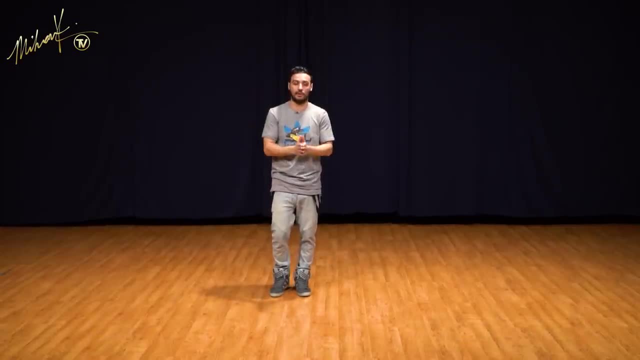 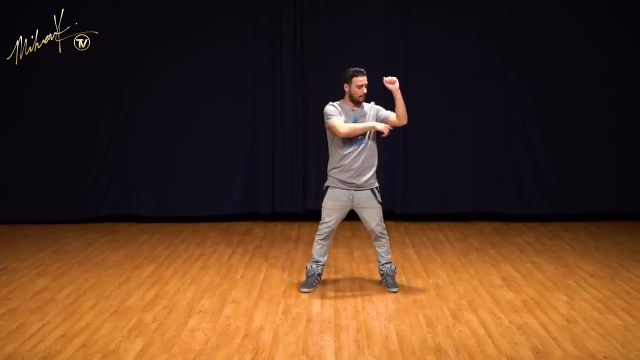 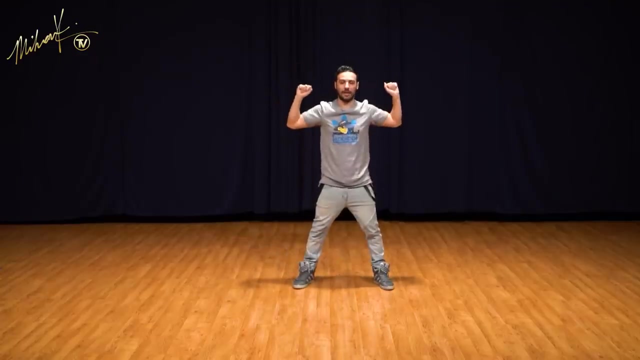 a smile in the first count. Going off of her lyrics, she goes: my smile is beaming. You're going to throw those hands, open them up, bring it back, Make sure you have a straight line, real sharp. Six, seven, eight and one and two. Good, One more time: Six, seven. 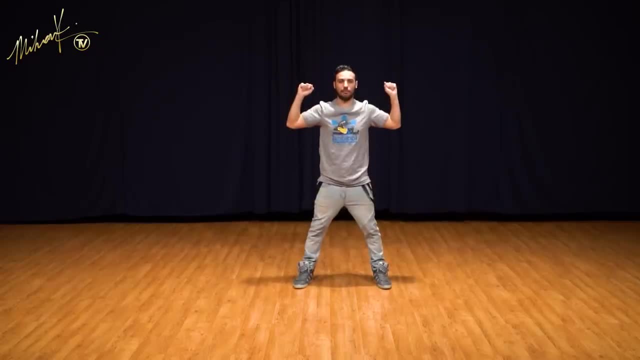 eight. my smile is beaming. Good From there. real sharp Fingers, open fingers, closed Hands are here. The right leg is going to go behind the left leg. The arm goes around My skin. Right hand here, open Left hand. you're going to make it a fist, You're going. 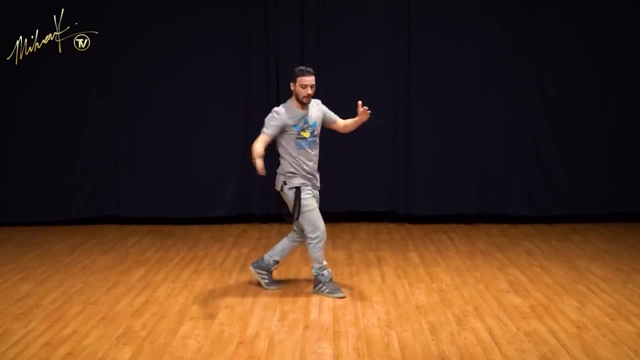 to go around the hand and stop. You want to use that right leg that's on the toes, That's going to spin you around. Still, keep your focus looking front One more time. You're going. my smile is beaming. You're going to go. my skin is gleaming, Going through the 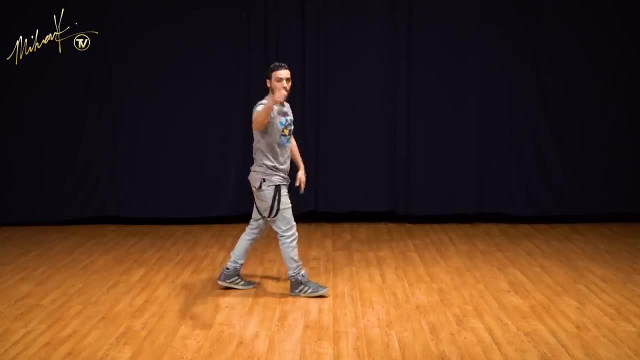 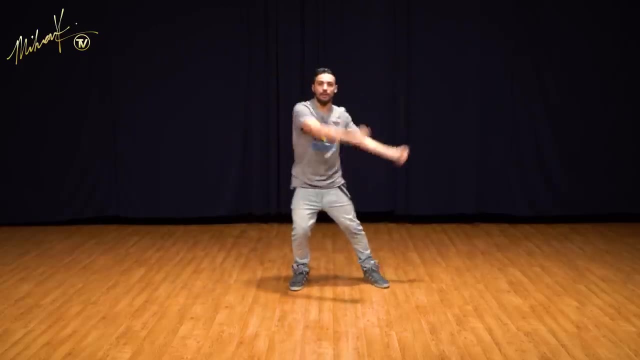 hand still up on the toes Right here, focus. You're going to go around the hand. You're going to focus to the front. Let's go from the top. Six, seven, eight. You go. one and two, three and four. Good, One more time. Six, seven, eight. my smile is beaming, My 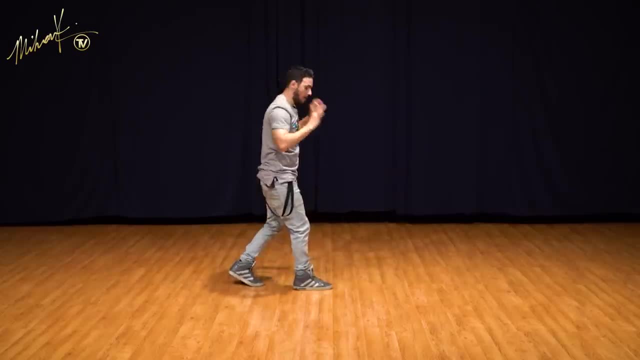 skin is gleaming Good. Have full control. Make it sharp One last time. Six, seven, eight. my smile is beaming, My skin is gleaming Good. From here, you're going to step forward with the right leg, Go in head first. You're going to do a body wave. You're going to say: 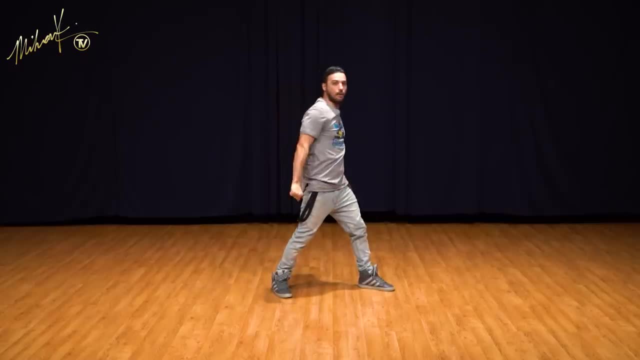 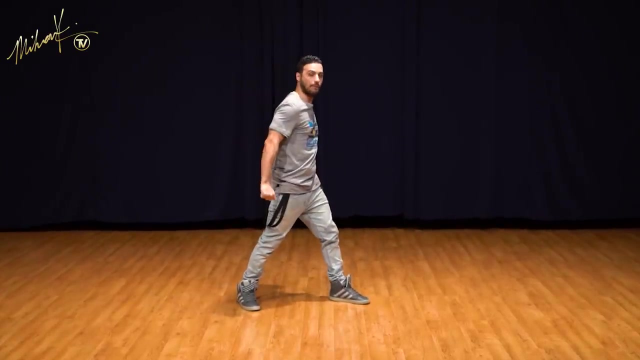 the way it shines, I know Good, Still keep your focus to the front. You're here. Six, seven, eight. The way it shines, I know. Come back really sharp on. I know. Make your wave happen on. shine The way it shines, Take it back, shines and boom, Come back really sharp. 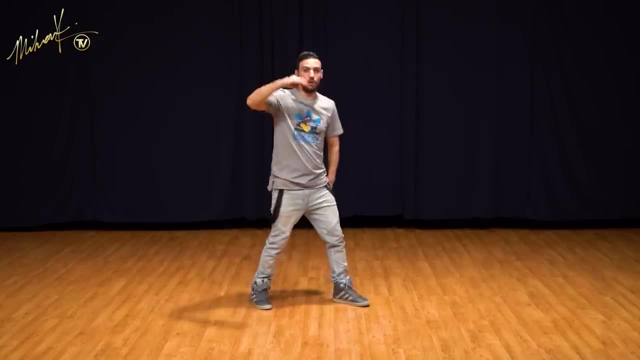 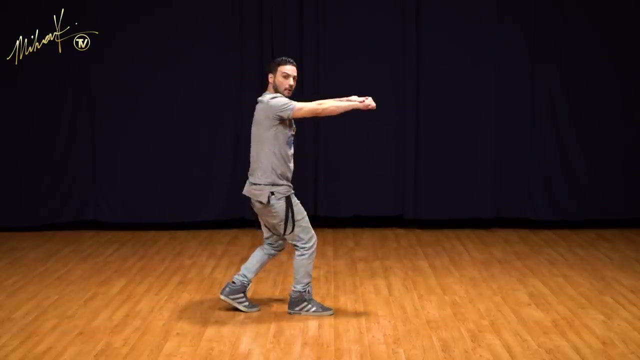 I know You see it Okay, So you're going to turn on you and then bring up the right arm on. see it? Good, Let's take it back and connect it from the top: Five, six, seven, eight. Go one and two, three and four. Go five, six, seven and. 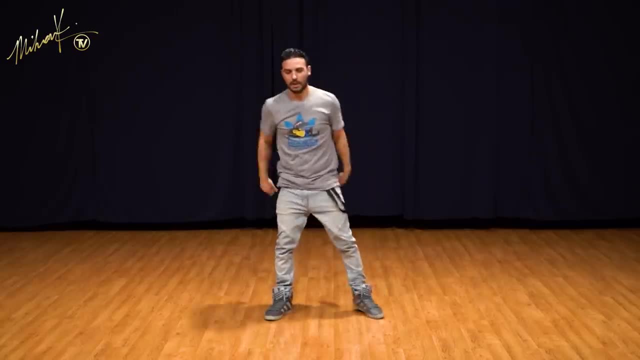 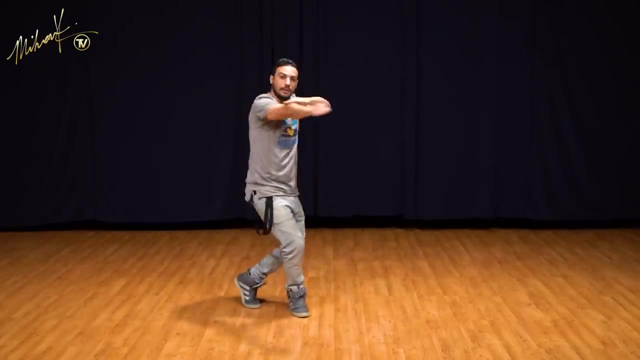 eight. Good, That's what counts, Left right. Okay, One more time with the lyrics: Six, seven, eight. My smile is beaming, my skin is gleaming. the way it shines. I know you see it. 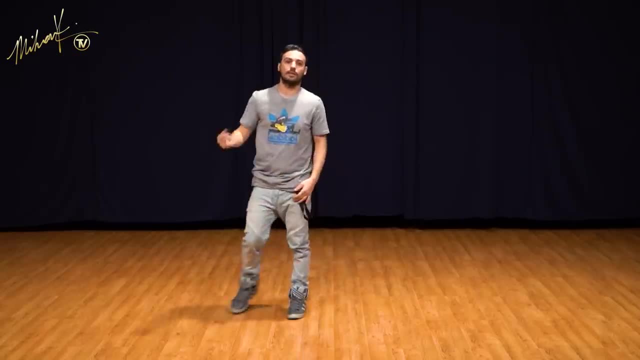 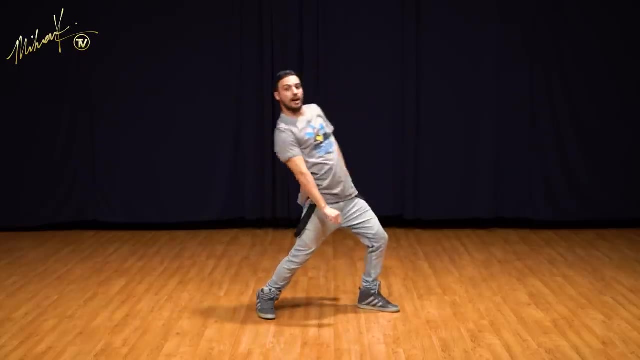 Good, One more time. Here we go. Five, six, seven, eight. My smile is beaming, my skin is gleaming, the way it shines. I know you see it. Good, From here you're going to go to the right side. small little bounce, use the left arm. 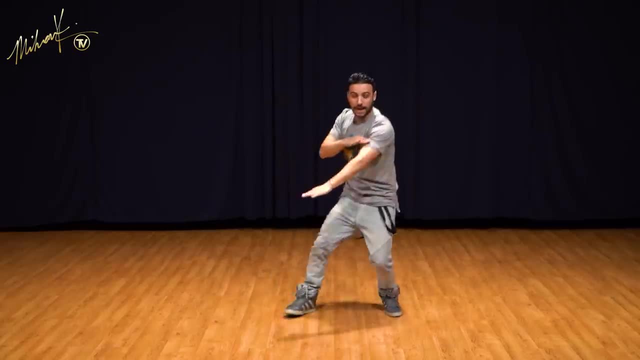 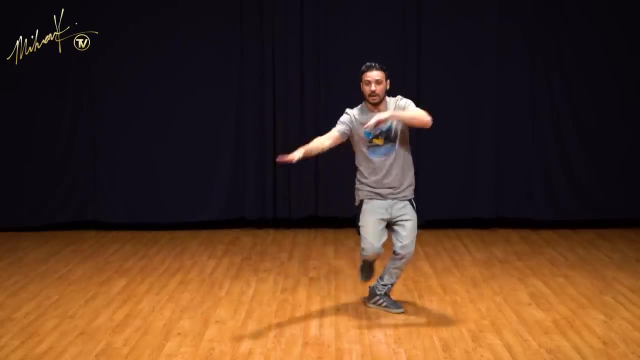 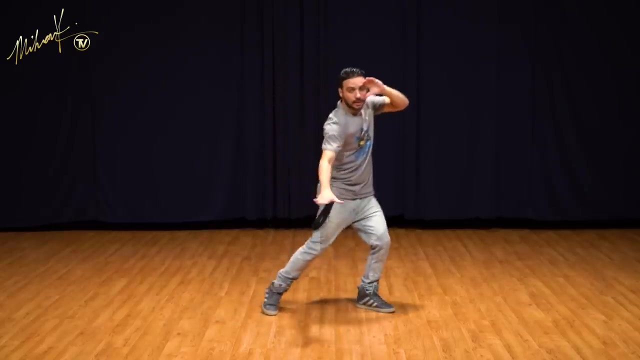 keep the right arm up. You're going to go bounce and bounce and cross. Okay, One more time. Six, seven, eight, I bought a crib just for. Okay, One more time. Six, seven, eight. I bought a crib just for. 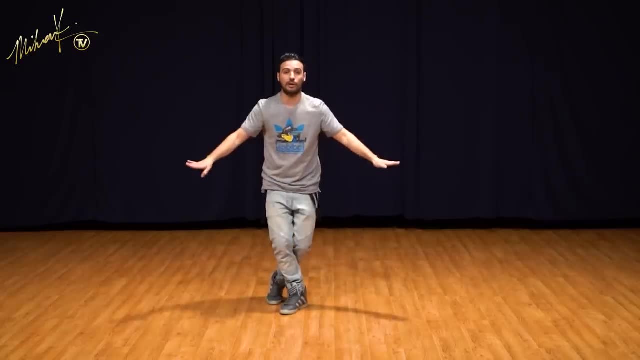 So I cross the arms first and then the right leg goes behind. Just for arms come together, the closet, And then you're going to open up. Okay, Just for The Closet. One more time, Just for The. 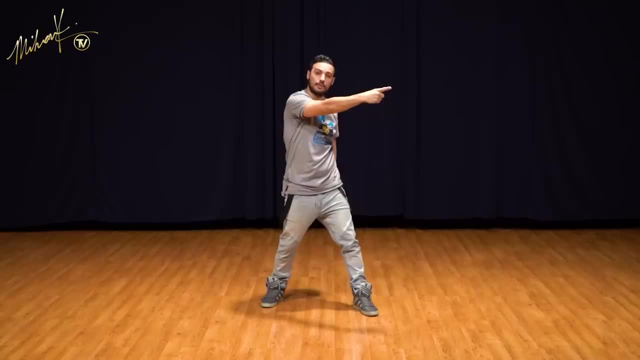 Closet, Okay. And then this part's pretty easy, Both his and hers. I want it, I got it, Okay. So you're going step and point. step and point, You're going to open up, bring your body forward, cross, hit the arms down, feet together. 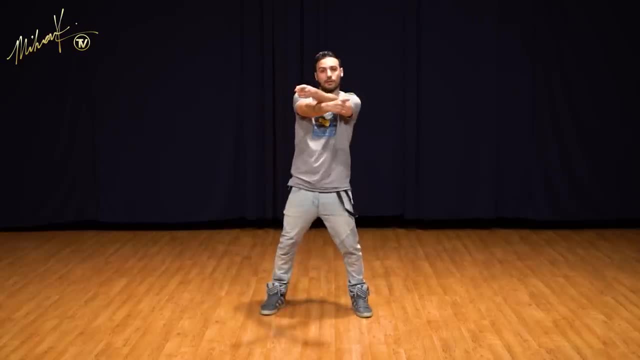 Okay, So lyric wise, Both his And hers. I want it. I got it Perfect, Let's take it back. Go from the top. So there were two eights in Almost there. Okay, Here we go. Six, seven, eight. 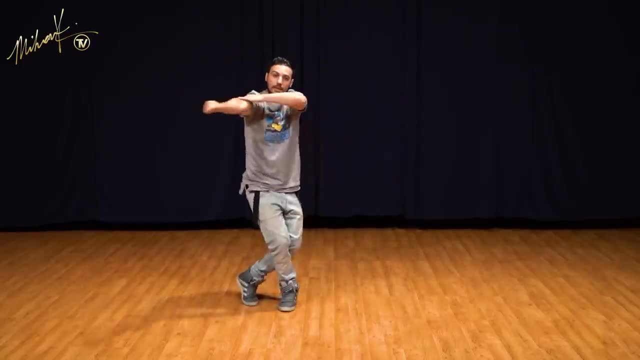 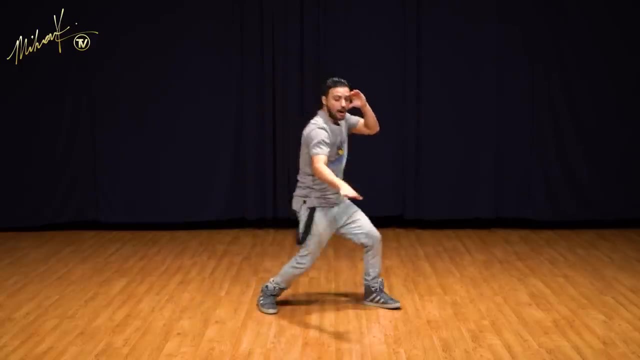 My smile is beaming. My skin is gleaming- The way it shines. I know You've seen it. I bought a crib just for the closet- Both his and hers. I want it. I got it Good. I don't think I've done this many lyrics in any of my tutorials. 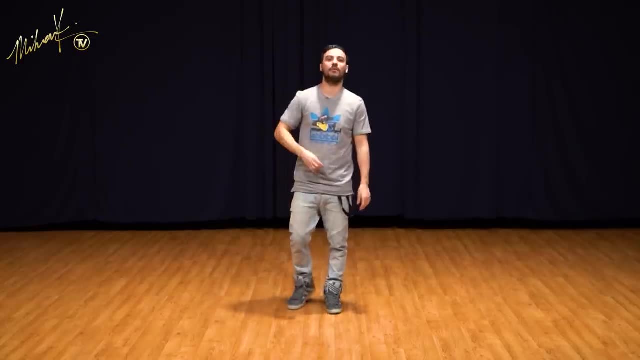 So here we go, Trying to break it down for you guys. Let's do it. We'll count some ones: Five, six, seven, eight, Go, one and two, three and four and five and six and seven and eight and one and. 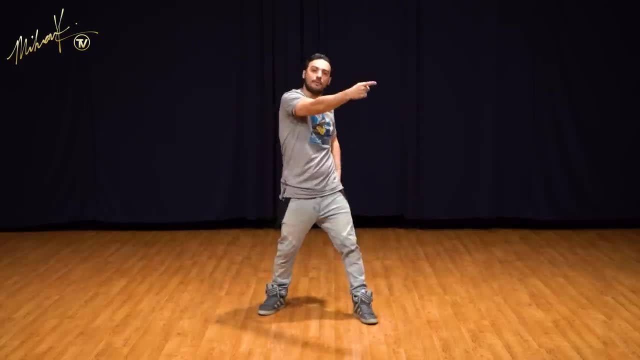 two and three and four Go five and six and seven and eight. Good. So if you notice, the steps are really really easy. Like I said, it's all about the timing and being sharp. If you could do it with the perfect timing and being sharp, it's going to look good. 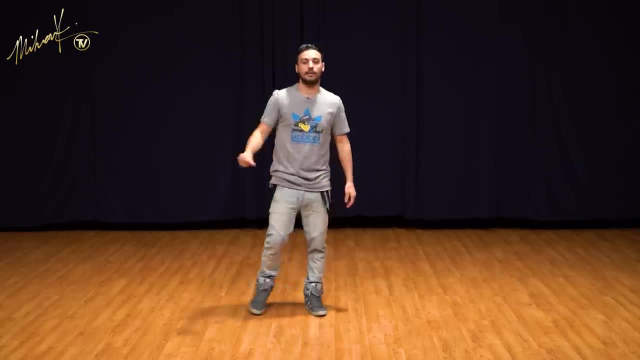 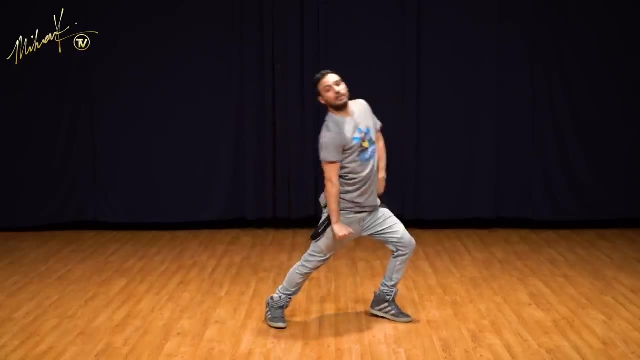 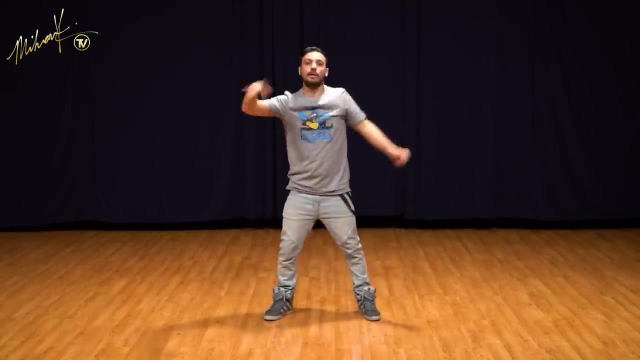 Okay, Here we go. One last time, Let's move on. Five, six, seven, eight. My smile is beaming. My skin is gleaming, The way it shines. I know You've seen it: I bought a crib just for the closet. 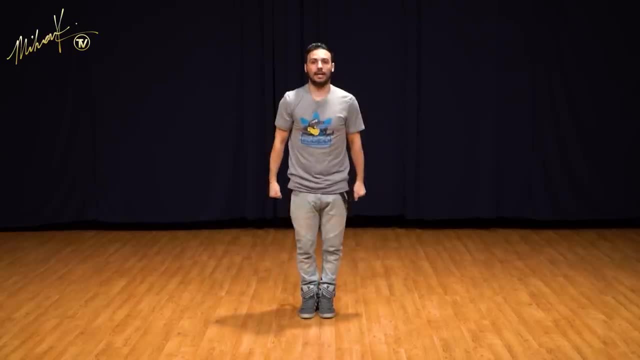 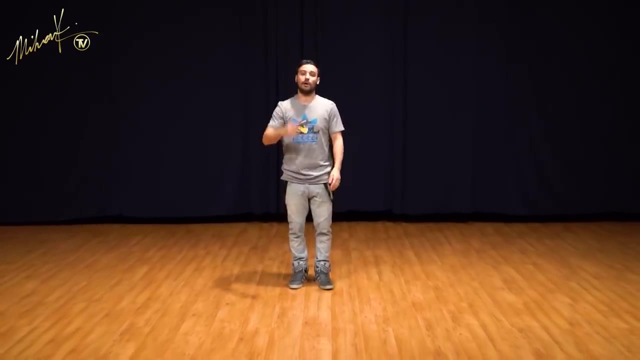 Both his and hers. I want it, I got it. Good, Let's move on from here. We're going to travel down, starting with the right leg. The legs are going to go right, left. The arms are going to go left, right. 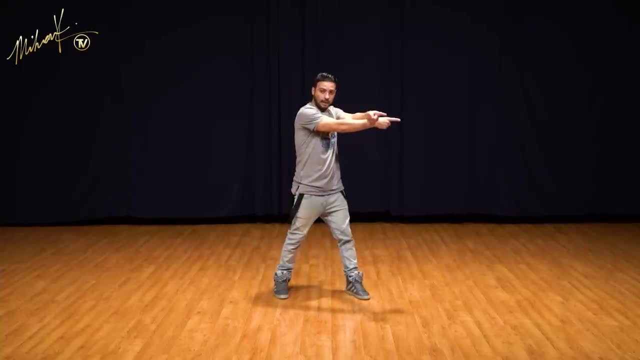 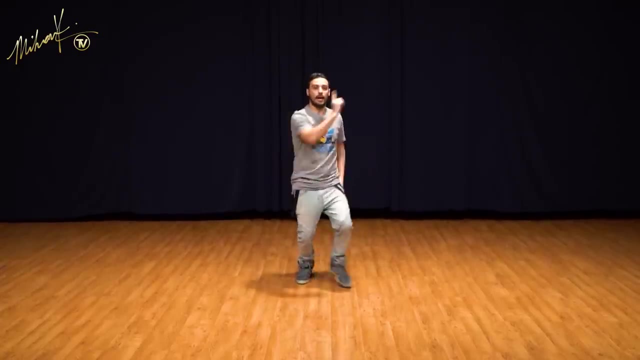 They cross Point point. So I want it Quick: hit with the head and then drop. I got it Okay. One more time: Six, seven, eight. I want it Hit. I got it Good. 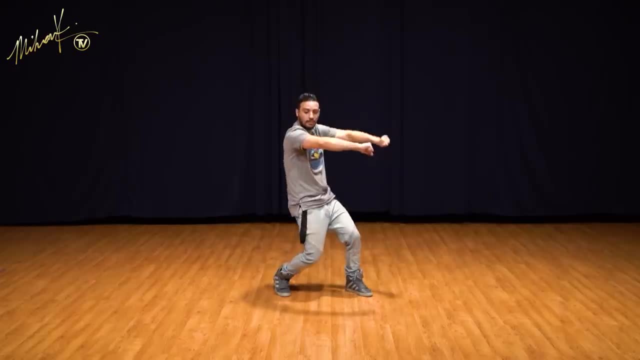 Again, Six, seven, eight and one and two Doing the same thing, going the opposite way. Make sure you step forward with the leg. Step forward with the left leg, first crossing the right arm. step, step, hit, drop, okay. 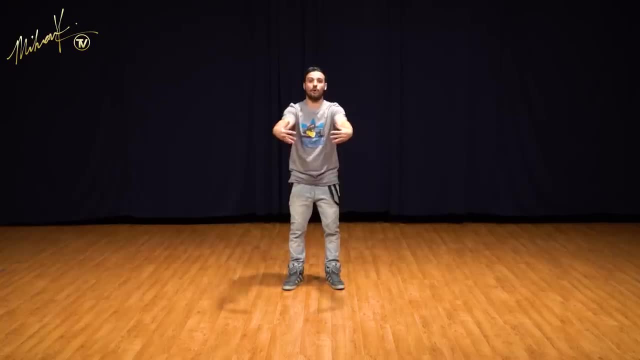 One to the right, one to the left. Do me a favor: Make sure you're traveling forward. Don't go to the right side and the left side. You're not going to the side, You're going down- Right, left drop. 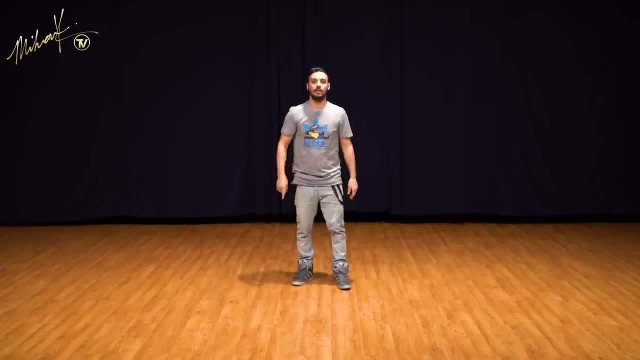 Left right drop. Okay, Here we go, Let's do it again. Six, seven. Your lyrics are eight. I want it, I got it, I want it. Hit, I got it. So you're squeezing that head in between. 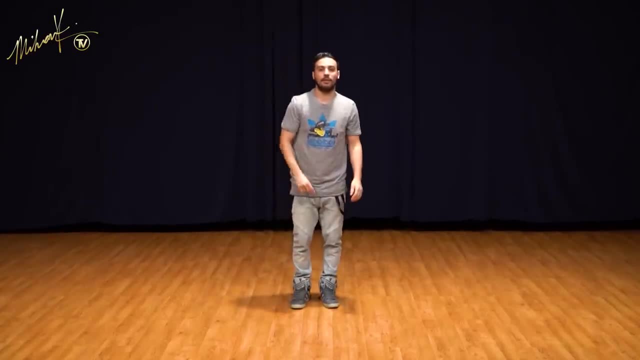 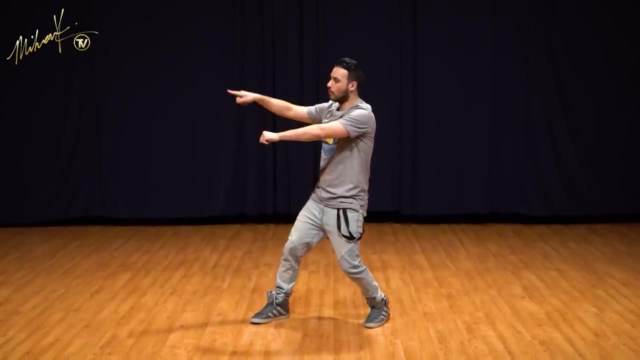 Okay. Between the lyrics: Five, six, seven, eight: boom boom hit drop. boom boom hit, drop. Okay, From here. this is easier. It's sliding over to the left side. Wave your arms to the right. 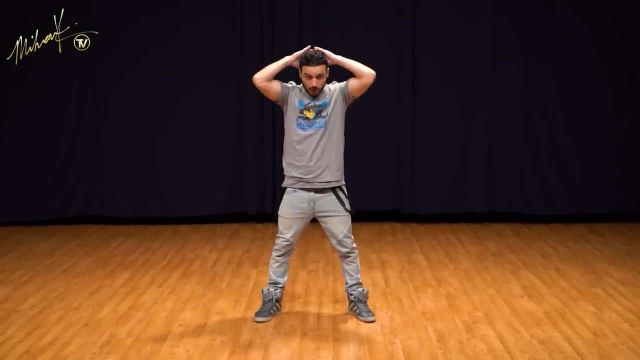 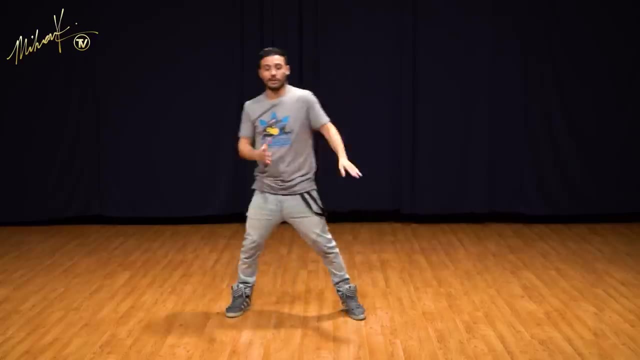 Go wave, wave, jump Arms, go behind and then you're going to go grab, grab, Okay. So when you do the wave, don't keep it simple, Don't just go slide, slide, Put a little like a quick, little, sharp, little hit to it. 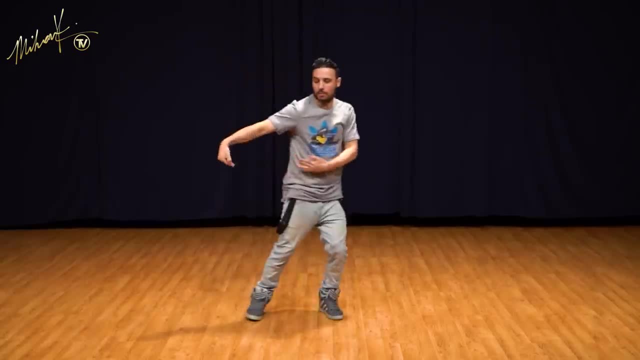 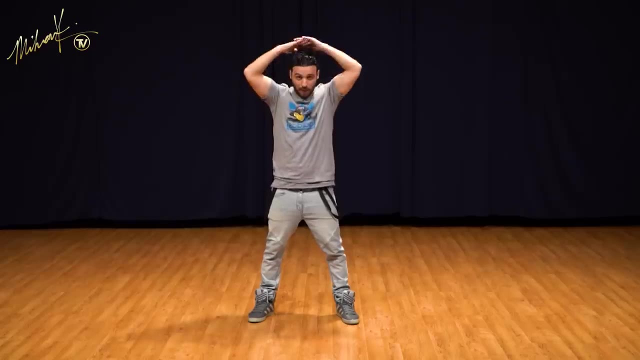 So it goes from fast to slow, Boom And boom. Same here. Jump, Step, step Good. So even though I jump and my arms go behind my head, it goes from fast to slow, Still moving, and then I go grab, grab. 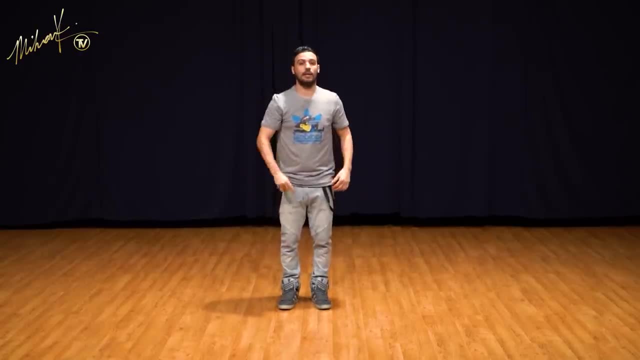 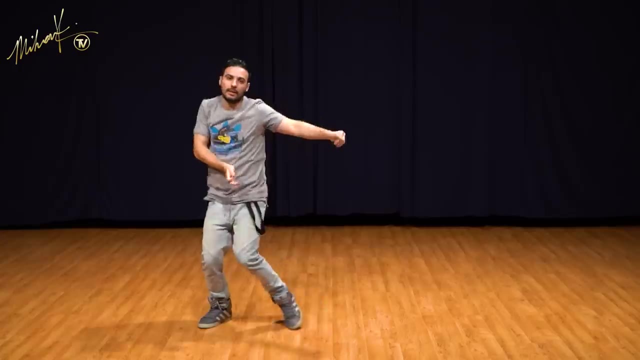 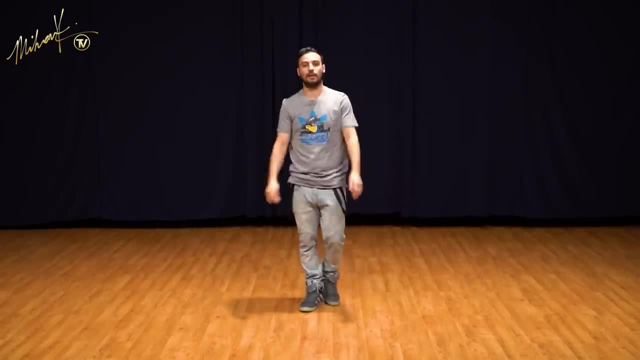 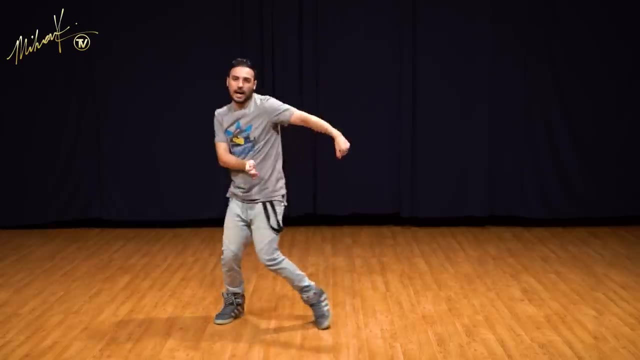 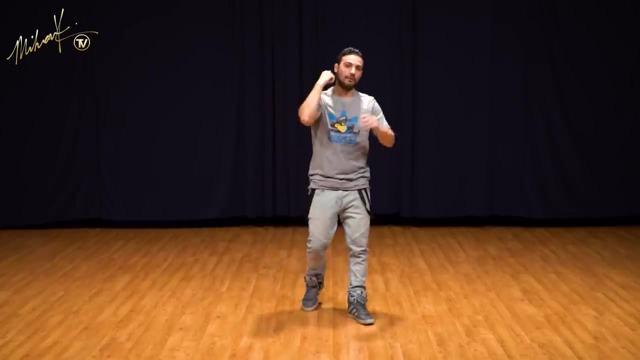 Okay, One more time. Five, Six, Seven, Eight And one And drop, And one And drop, Go, slide, Go, slide, Go, boom, Hit, Hit, Nice And the arms go right, left, Okay. 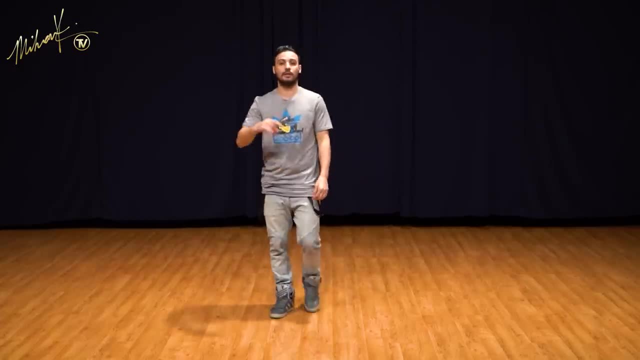 Let's go back from the top. Let's connect it together. We're almost done From the very top. Here we go: Five, Six, Seven, Eight. My smile is beaming, My skin is gleaming, The way it shines. 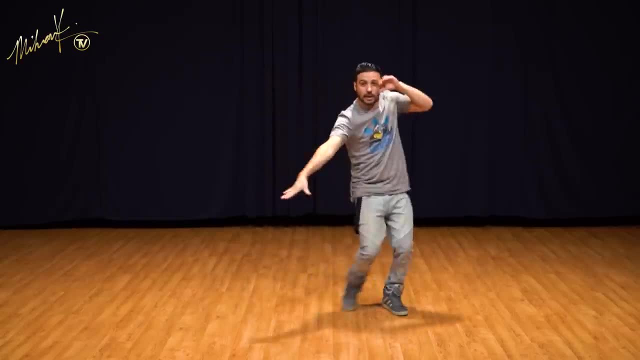 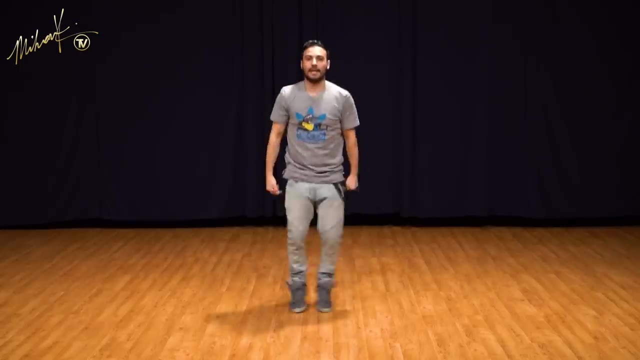 I know You've seen it. I bought a crib just for the closet, Both his and hers. I want it, I got it. I want it. Hit Got it. I want it, Had, Got it And boom. 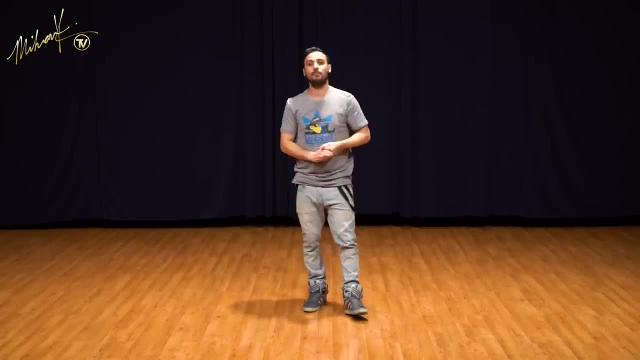 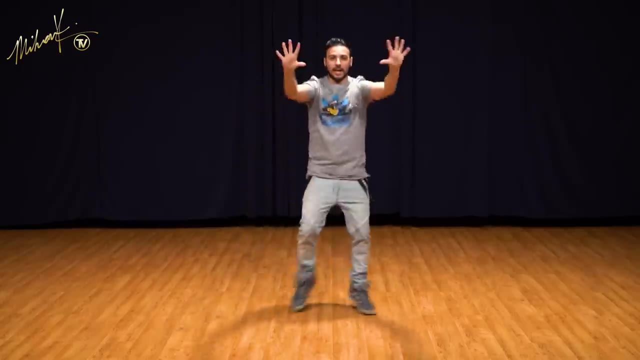 And boom And jump, Boom, Boom. Good, Let's try that one more time. Yeah, Slow it down a little bit, just to clean it up. Five, Six, Seven, Eight And one And two And three. 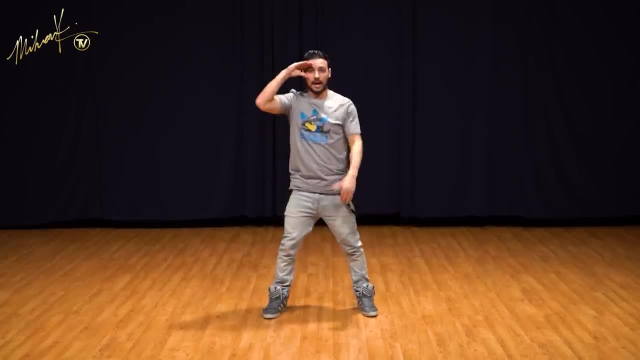 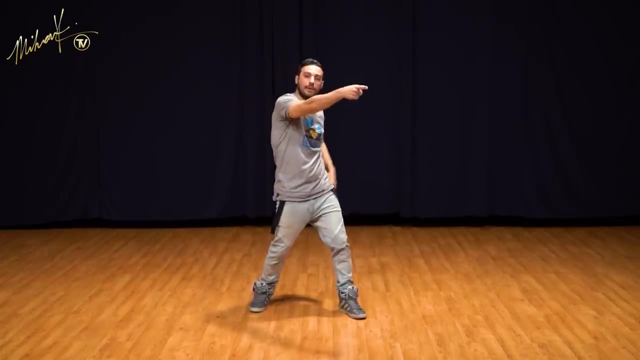 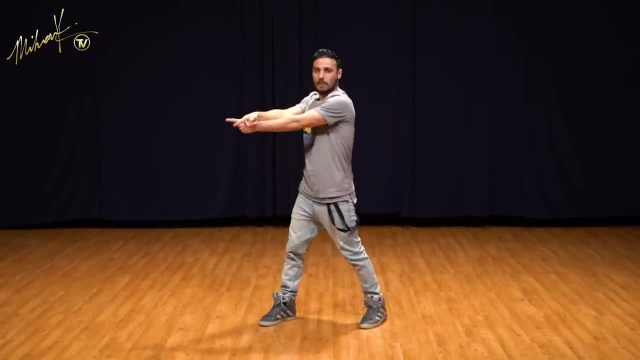 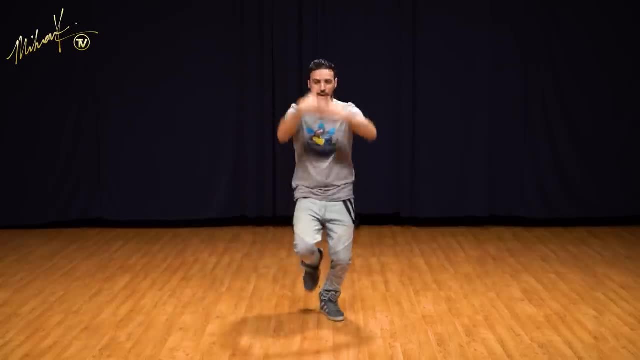 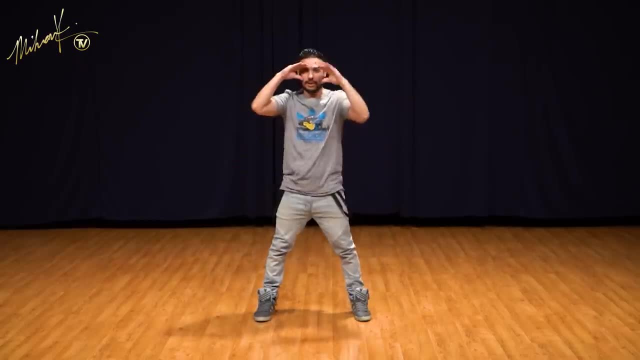 The way it shines. I know you've seen it. I bought a crib just for the closet, Bought his and hers. I want it, I got it. I want it, I got it, I want it, I got it. Go hit. 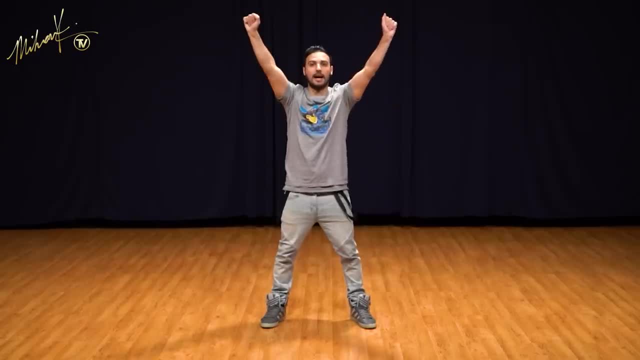 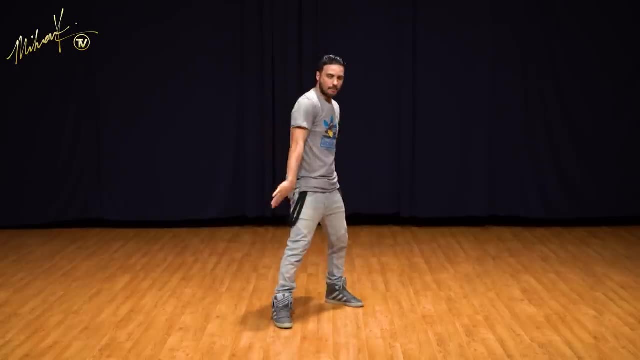 And hit And boom Tha tha Good. From here you're going to step back with the right leg. body's really stiff, the arms are really smooth, So your leg is go, step and step easy. six, seven, eight, right leg, left leg- okay. 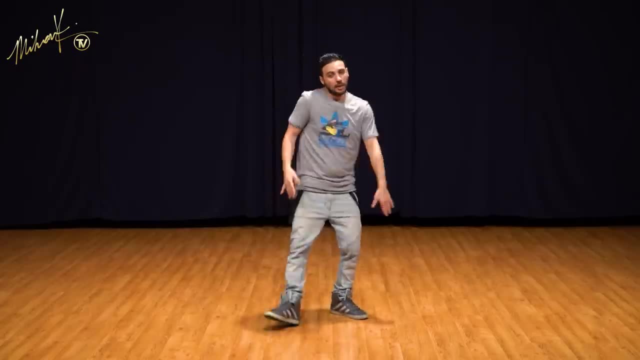 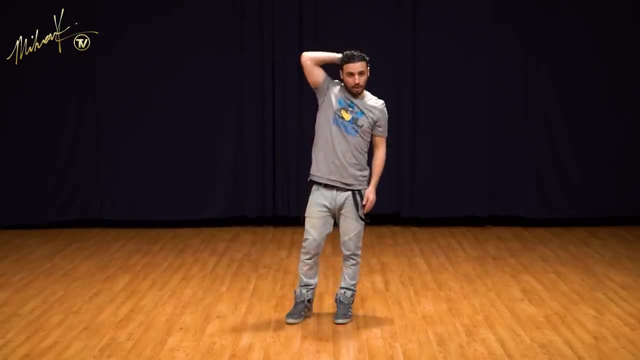 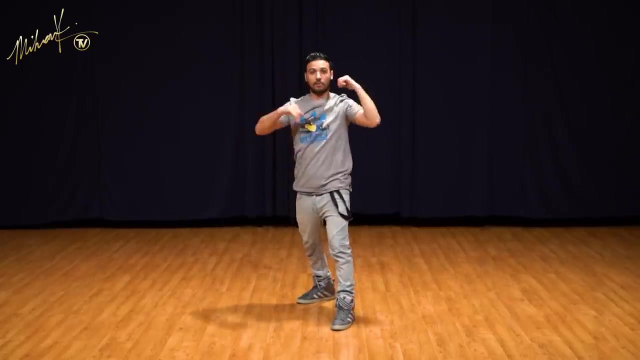 You turn to the right, you're facing the right, boom, boom. okay, Arms, you're going. you like my hair? okay, Left arm, right arm moving. six, seven, eight, You like my hair? you're going to go. gee, thanks, just bought it okay. 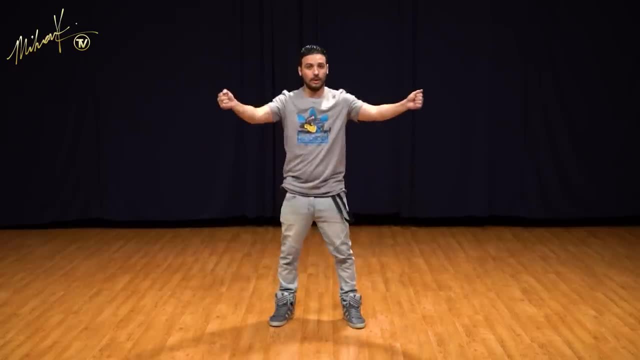 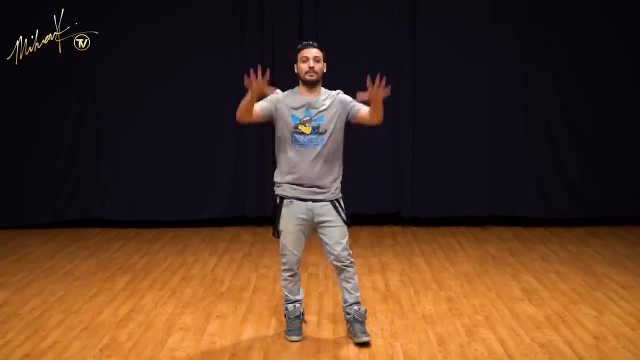 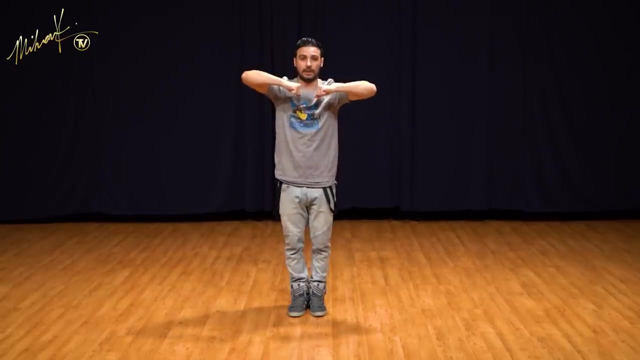 So if you remember before that we went: boom boom, boom boom, arm leg, arm leg, same thing here: arm leg, arm legs. okay, So go from here. seven, eight, you like my hair? arms jump together, arms cross make. 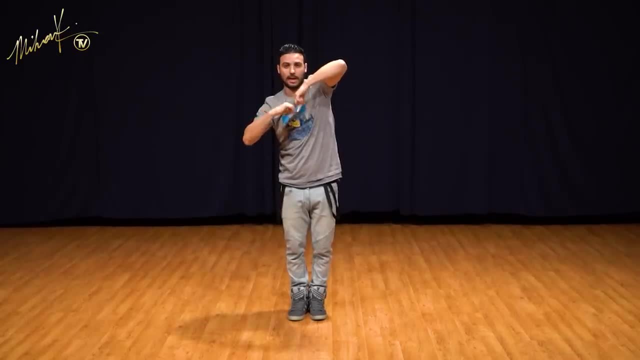 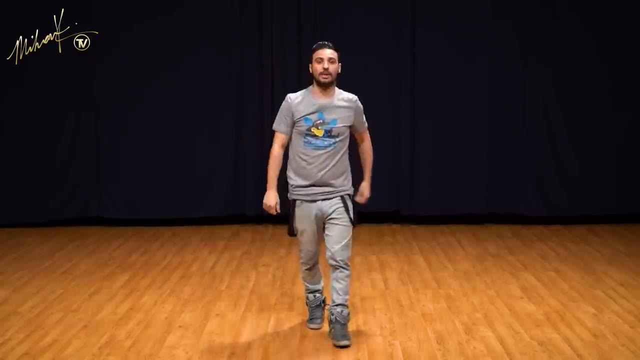 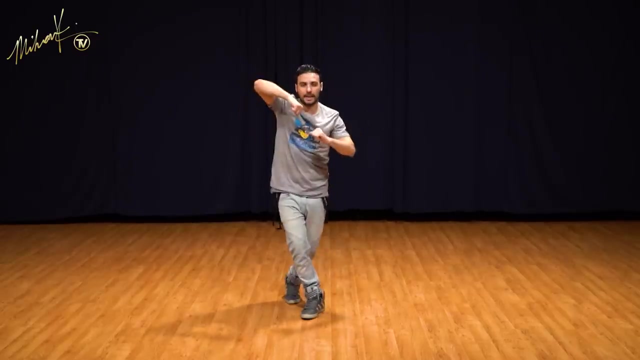 sure you're still keeping a good line here. Fist really sharp, Don't be lazy with the hands. okay, boom, face it over. cross the legs, left leg crosses in front of the right leg. okay, One more time. six, seven, eight. you like my hair, gee? thanks, just bought it. 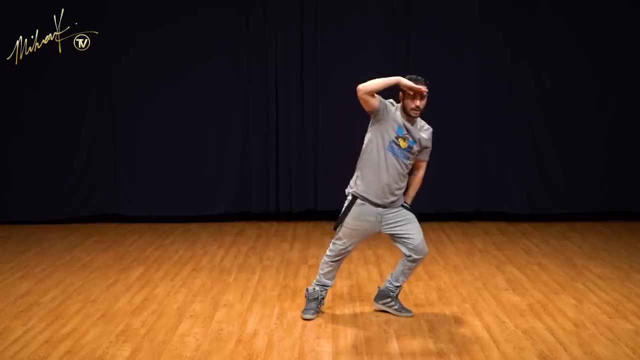 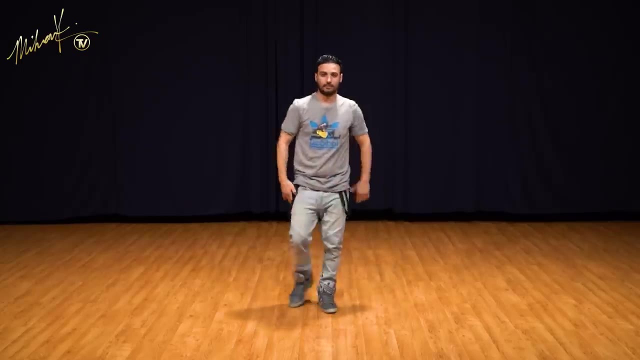 Let's finish this part up. this is easy. You see it or I see it. I like it, I want it. I got it easy right. So you're here. right here, put all that weight on the right leg. 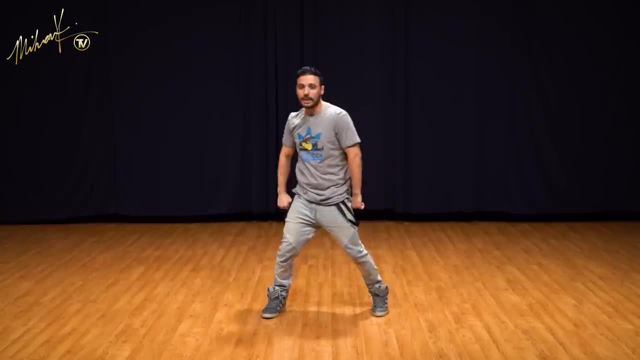 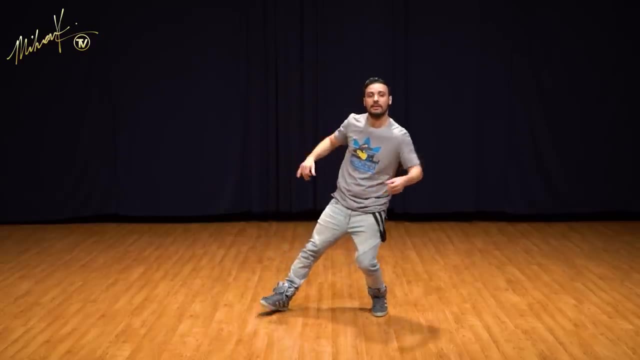 I see it. You're going to look, nod your head. I like it moving on, transferring your weight to the left side, okay, and then you're going to say: I want it use your hands. the head still nods. I got it slide back with the left leg, throw the arms, small little slide. 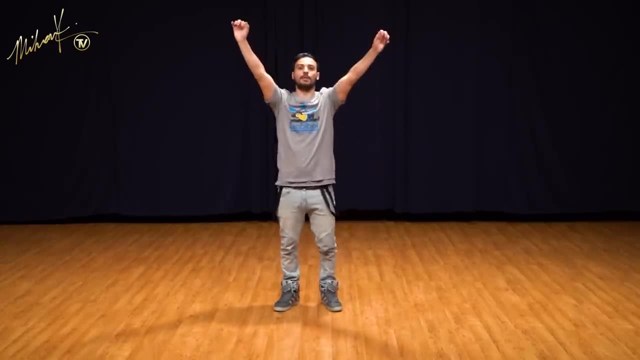 to the back and that's it. okay, guys, Let's take it back from here. six, seven, eight, you're going. you like my hair? gee, thanks, just bought it. I see it, I want it. 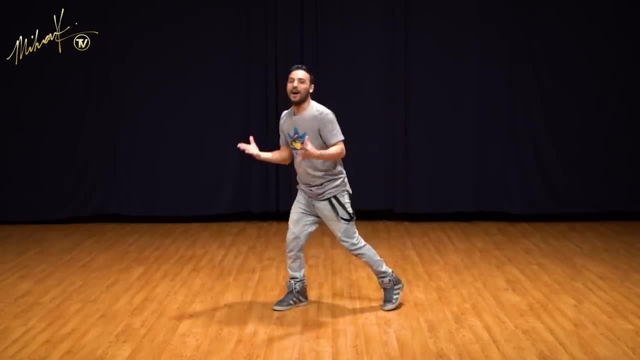 Oops, sorry You're going. I see it, I like it, I want it, I got it. I'm surprised. I even know the whole lyrics. okay, Here we go. let's take it back to the top. that's the full routine. really, really simple. 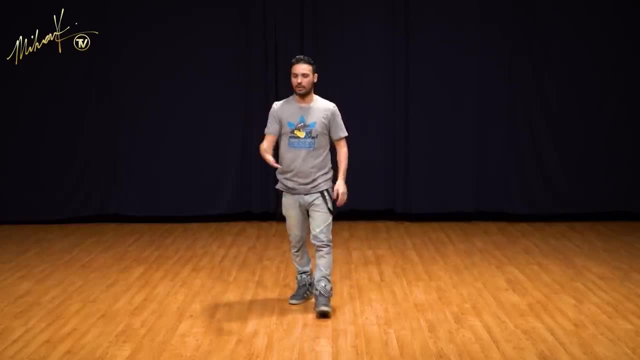 like I said, this is a beginner routine for kids. I taught it to all the kids in my class. really simple, all about the timing and being sharp. steps are simple. I feel like you should be able to do it. just keep doing it and again if you feel like it's still too much. 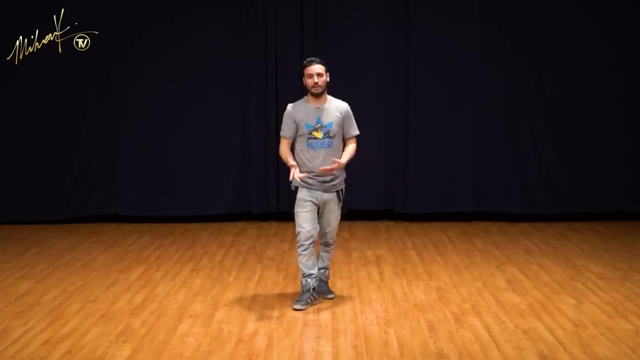 watch the video again and then do it again, because you're trying to learn it in 10, 15 minutes. That's the whole class. okay, Let's take it back from the top. let's do one: super slow, medium tempo, full tempo. 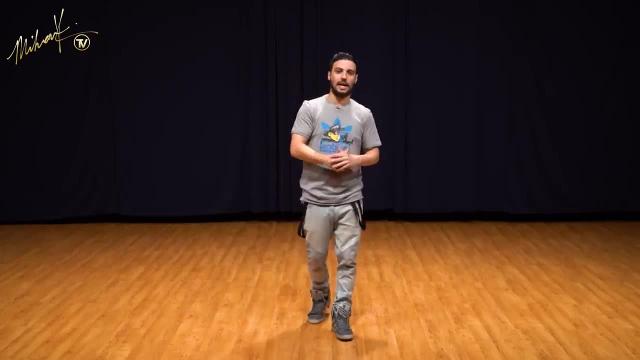 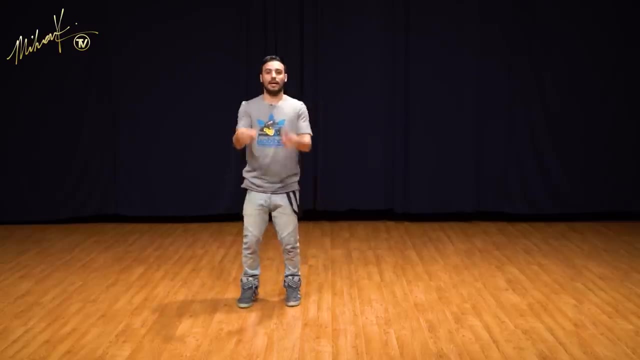 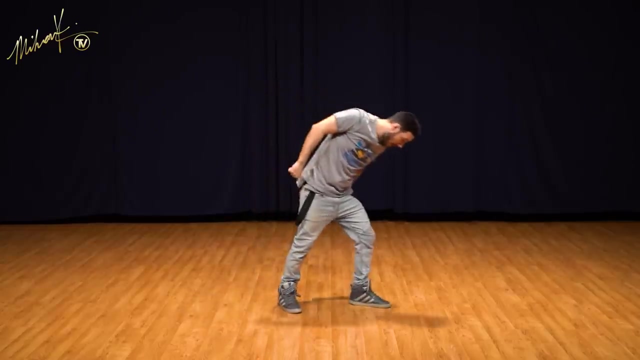 and then the dance video link will be in the description box. you can watch the video again and go ahead and do it along with us. okay, Here we go from the top. slow, five, six, seven, eight, Hit, drop, step, step, hit, drop, go, slide and slide, and slide and hit you.